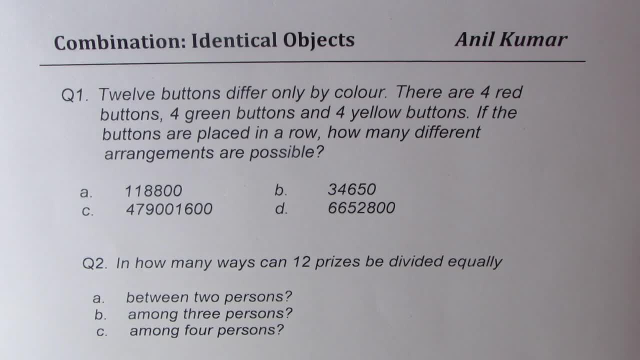 between two persons, among three persons, among four persons. You can pause the video, answer the question and then look into my suggestions. Now let's see how to solve such questions. In the process of solving this question, I will also share with you a method which will 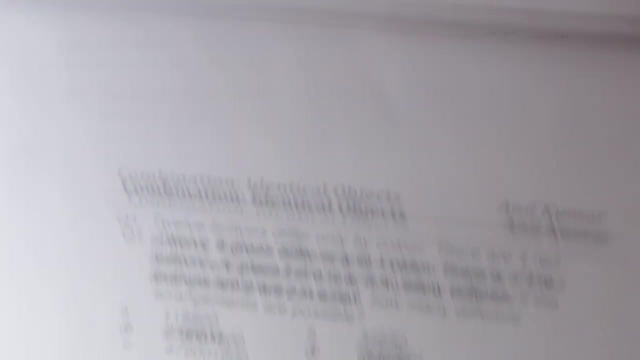 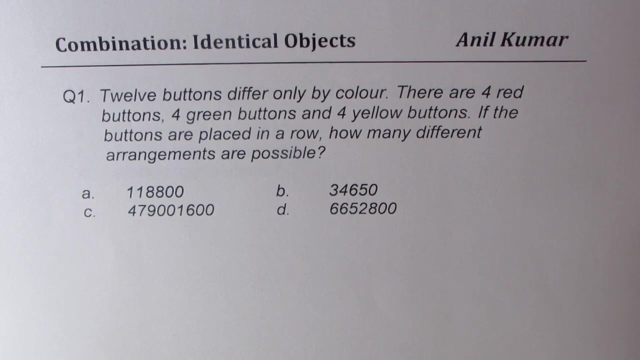 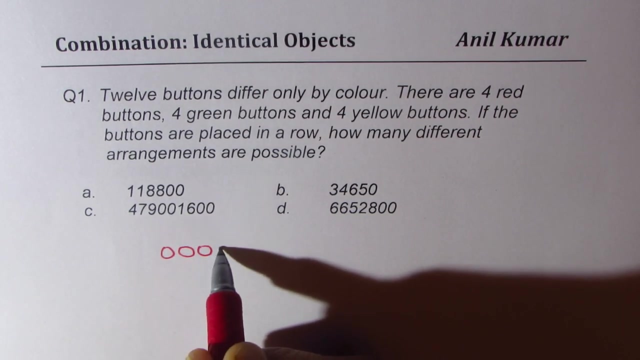 help you to solve all similar questions. Question number one: We are now talking about twelve buttons which differ only by color, So there are four of each kind, right? So we have four red, for example, and we have four green and four yellow. So we have four green. 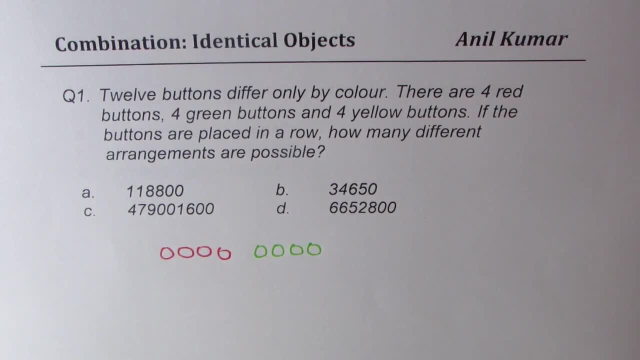 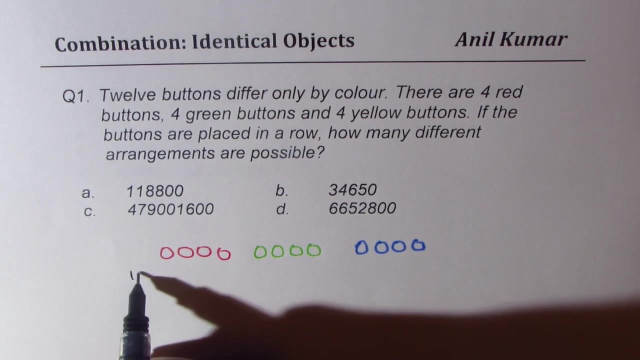 And for yellow, I'll just put blue color. Now they are exactly similar except for the color. Now you need to find how many different arrangements are possible. So the clear answer here is that there are twelve in all. so twelve factorial divided by four, of each kind are same. So those are the twelve buttons. So 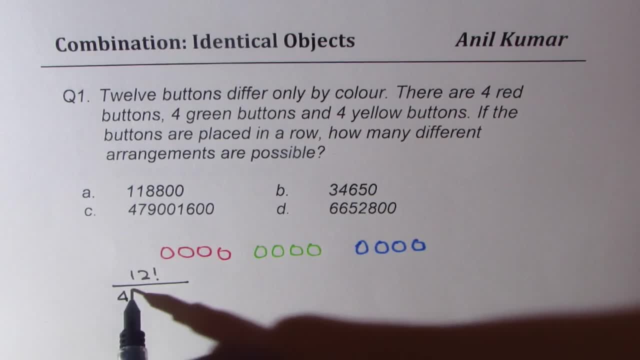 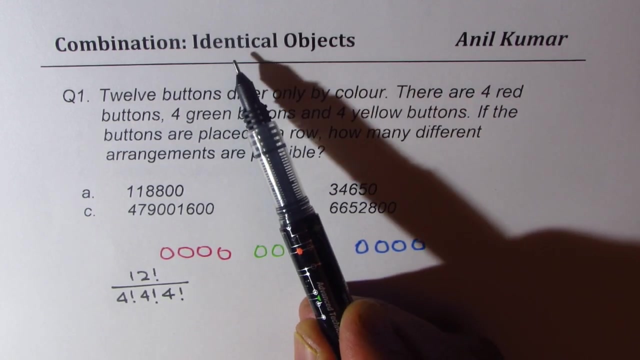 those combinations will be similar. So we need to divide by four factorial For red, four factorial for green and four factorial for yellow, which are shown as blue. So that becomes our answer. Now, this is one approach which we have learned for identical objects. 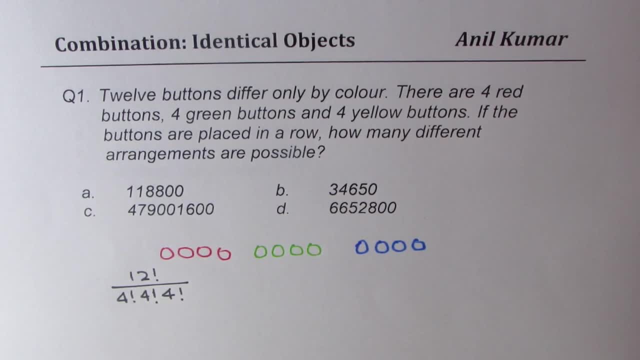 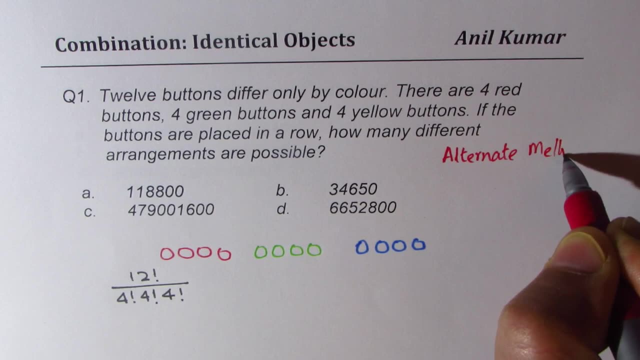 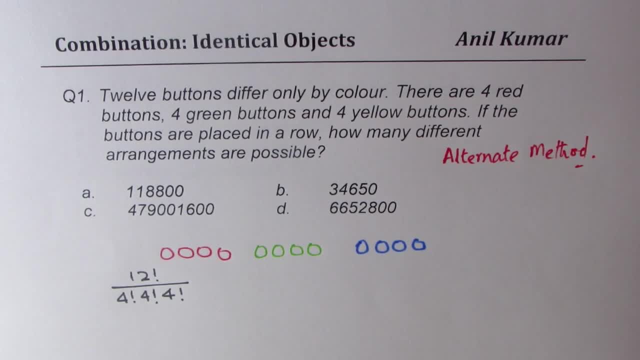 purpose method which could be used in many such scenarios, and that is why I am discussing this now for question number one, and it is going to help us to solve question number two and similar examples. So the question again here is that we have twelve of these right, So what we should. 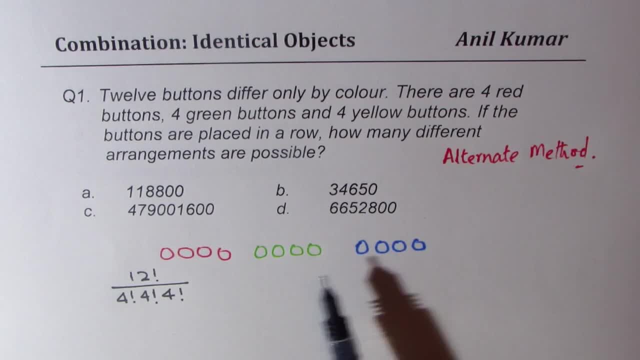 figure out is that how many arrangements are possible to distribute four of one kind out of these 12.. So if we try to select four red ones, then out of 12, we are selecting these four, So we get a choice of 12C4.. 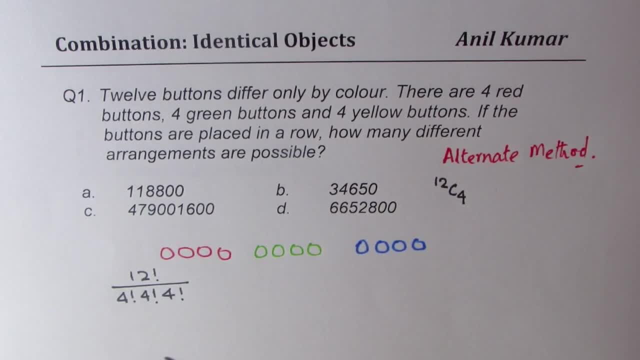 Now, once we have distributed these four, then let's think about distributing the next color. Now, that next color could now be distributed from eight of these, So that means from eight. we are selecting again these four greens. Now, whatever left is to be distributed. 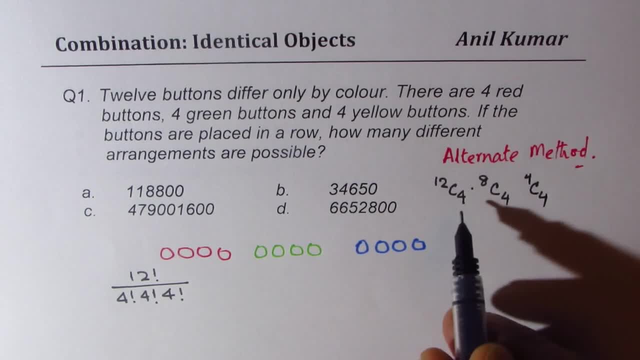 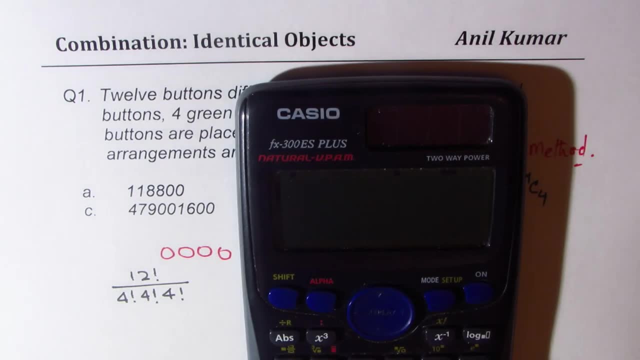 So it is 4C4.. So that is alternate way of doing the same thing, Correct? Let's figure out both the answers right. So we have 12 factorial divided by so within brackets, let me write cube of 4 factorial, which is cube of 24, right? 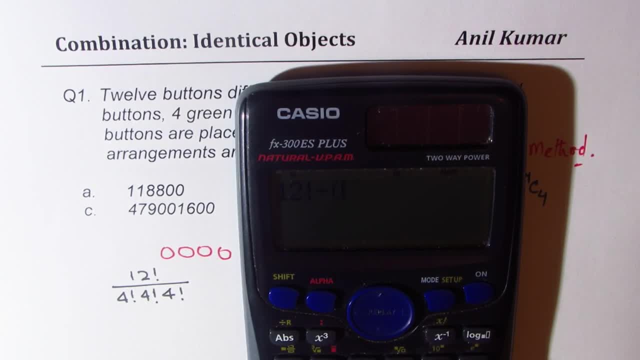 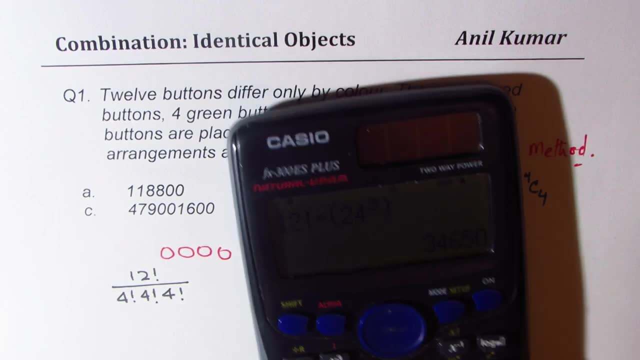 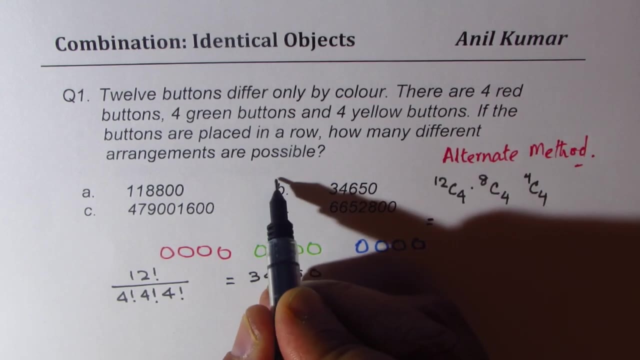 4 times 3, 12.. 12 times 2 is 24.. So let me write 4 cube here and equals 2.. It gives us 3, 4, 6, 5, 0.. So option B is the right option, correct. 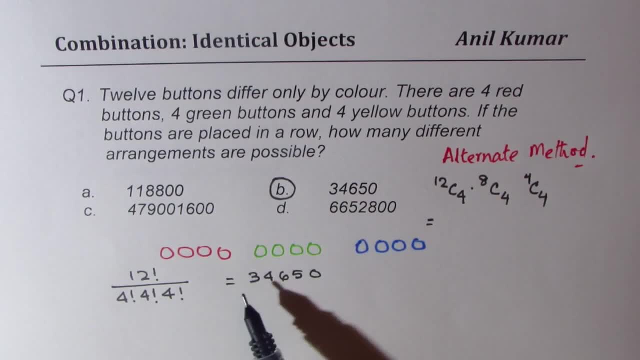 Now, this is not a very difficult question. This is straightforward, many of you know. However, the method which I'm talking about is very useful. Let's try to calculate this value also. So what we have here is 12C4.. 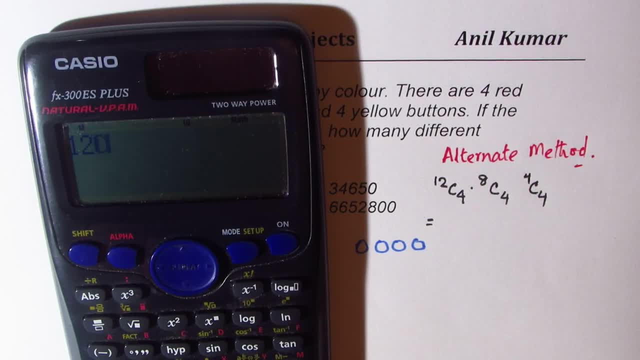 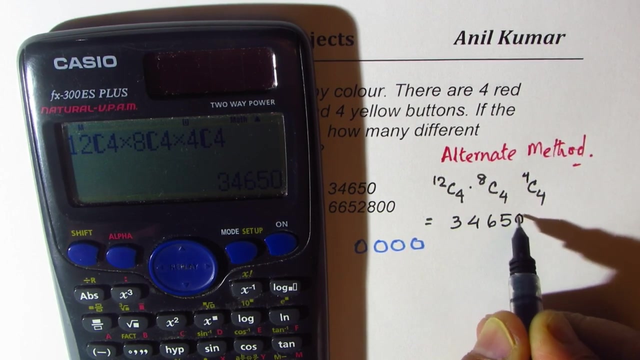 So we have 12C4 times 8C4 times 4C4, which is 1,, of course, And what do we get? We get the same result, which is 34,650.. Do you understand the method? 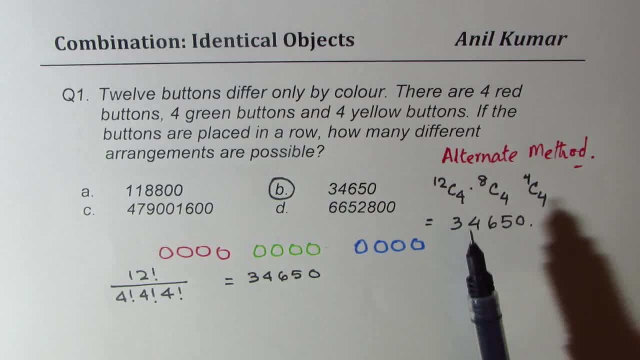 So what we have done here is that we are now thinking about first distributing these four, then those and then the next lot, So in this fashion we can actually deal with identical objects with just combination formula, as we did now. I hope that makes sense, right. 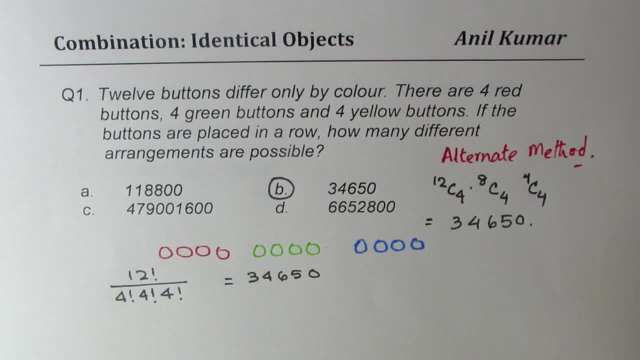 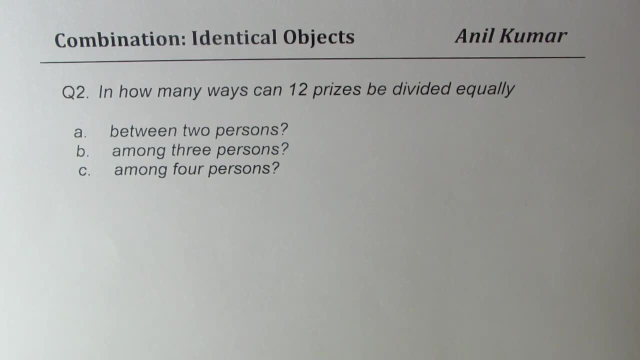 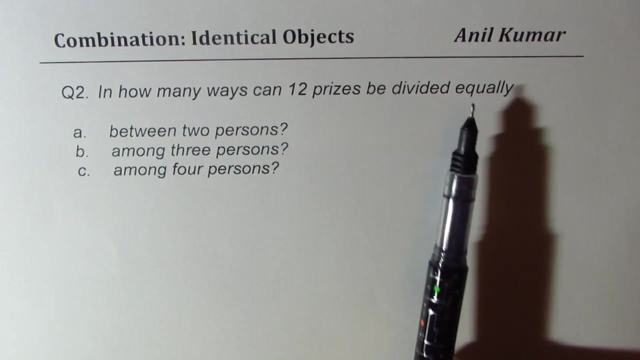 Now the answer is clear. Let's get to question number two and see how our method helps to answer such questions. Now. question number two is: in how many ways can 12 prices be divided equally? Now, when you divide prices equally between two persons? 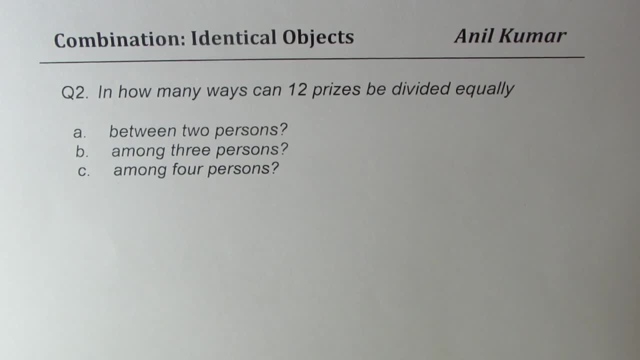 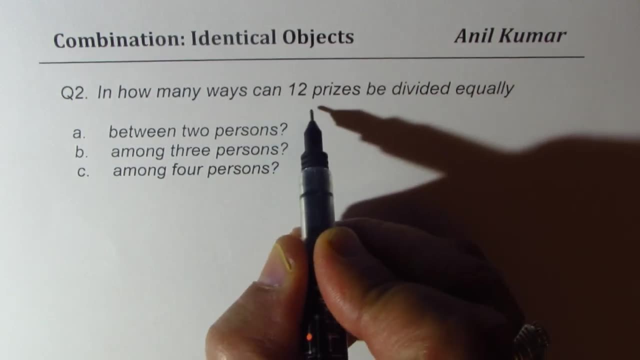 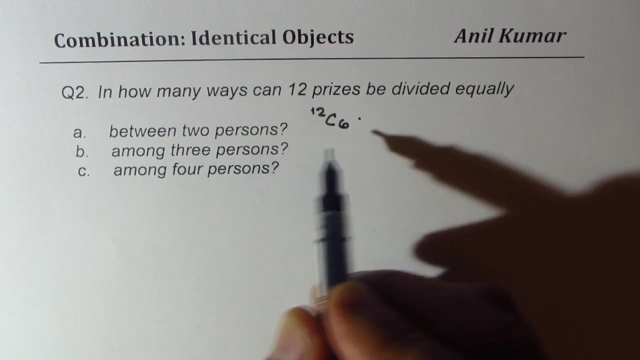 then each is getting six correct. So that means that two persons. so to the first person we have to give six prices, So that is from 12, we have to choose six. And to the next person, six out of six, right. 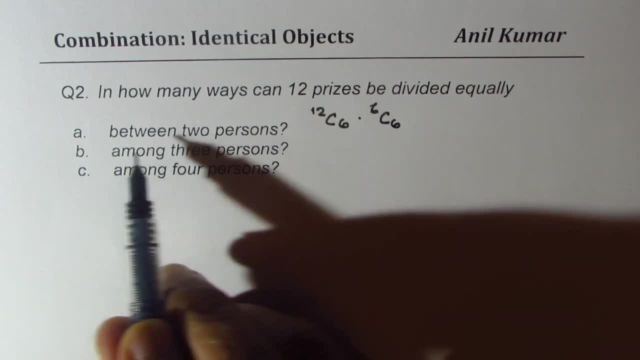 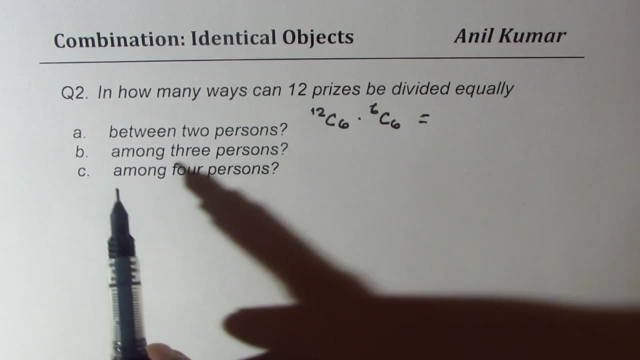 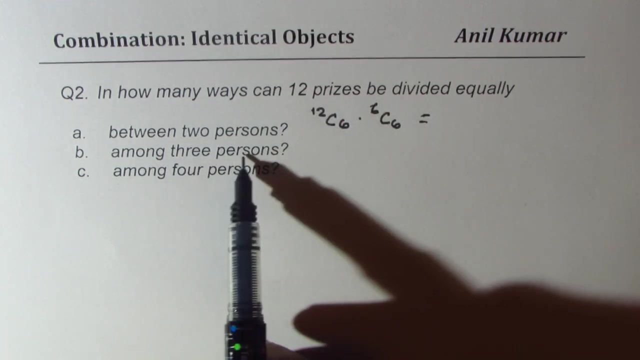 So all other six goes to the next person. So that becomes the answer for part A, right? So you can always calculate this. You get an idea, right. Question number two is to select to distribute 12 prices. so 12 prices among three persons. 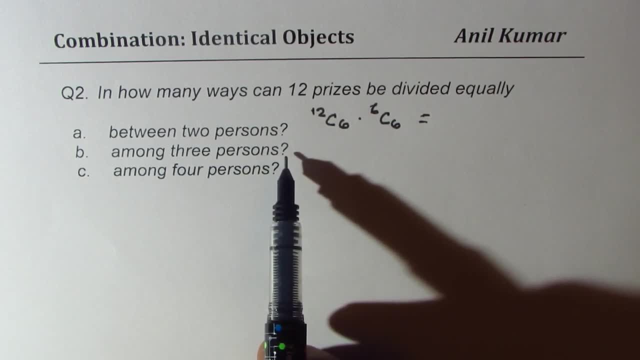 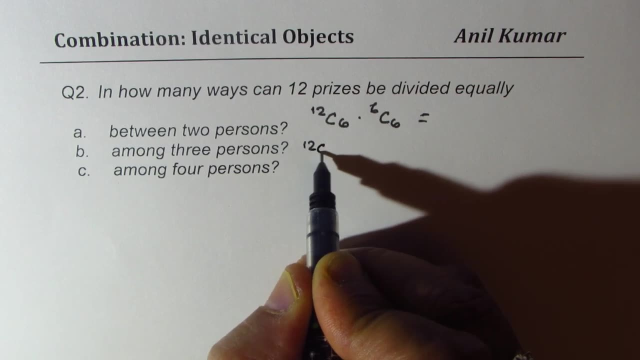 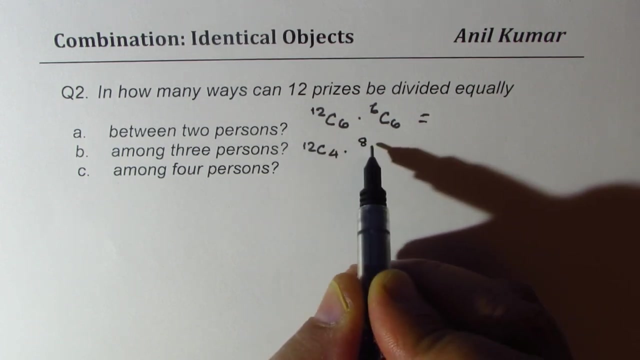 Among three persons means everybody gets how many? Everybody gets four each right, So this should be from 12, let's collect, select four. Then for the next person we have to choose from eight, since four have been given out. 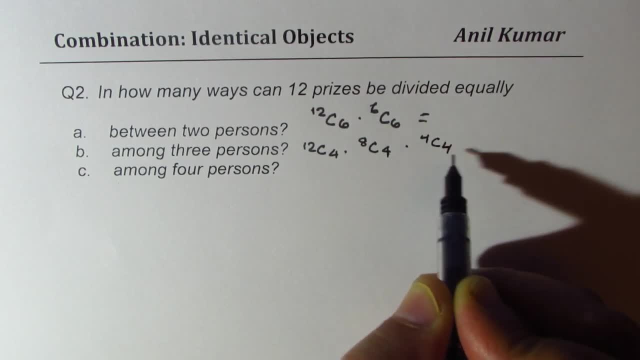 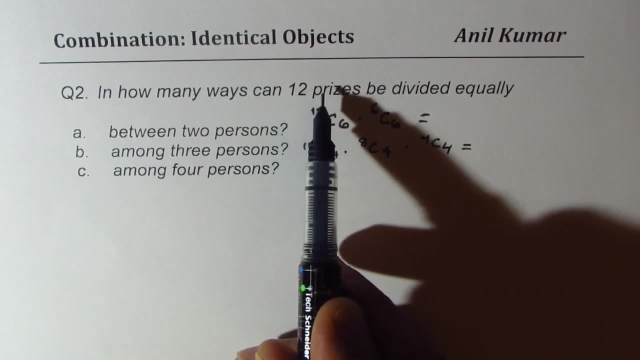 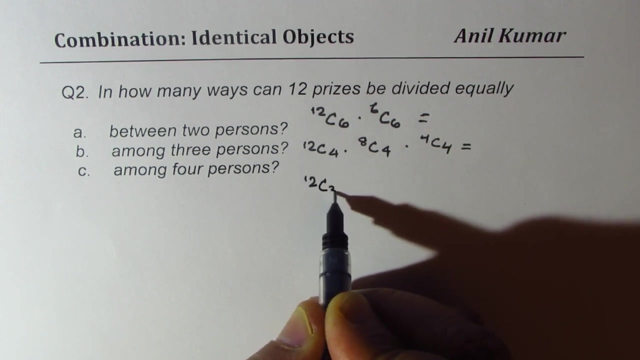 four, and then we have 4C4.. That becomes the answer perfect. And the last one: if there are four persons and there are 12 prices, each gets equally how many Three right? So here the combination is 3C3 times. 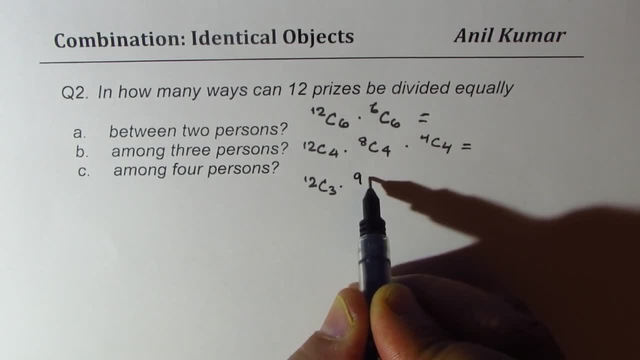 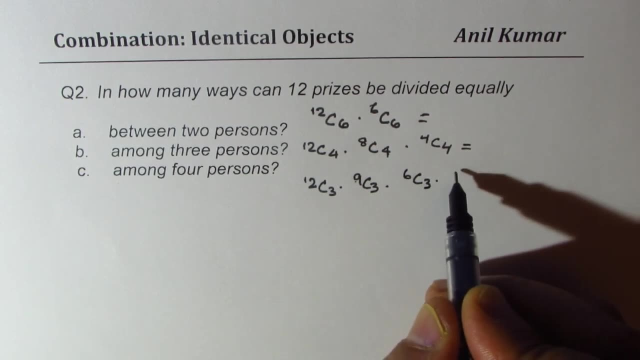 take away three, we are left with nine right, So 9C3, and then we take three more, we are left with six, 6C3 times 3C3.. Do you see how we can collect the answers? 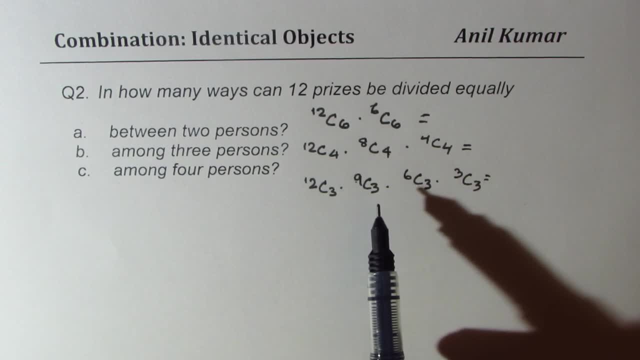 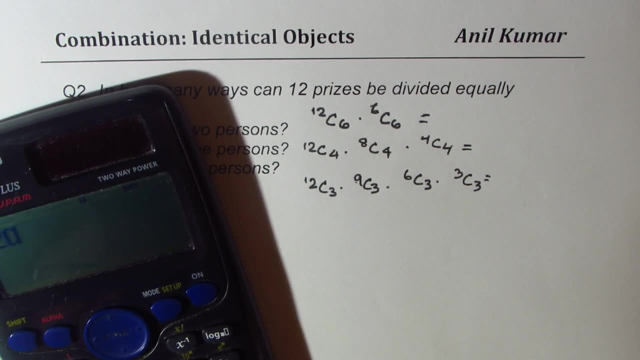 Very easily using this concept: Perfect. Let's calculate the answer. So it is 12C6 for the first one, which is equal to 924.. For the next one, it is 12C4 times 8C4 times.